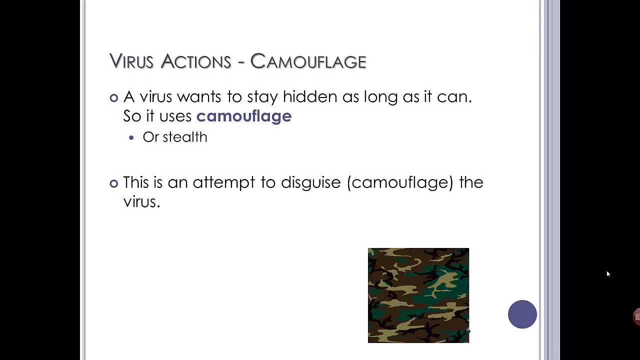 the immune system will attack it. you employ antivirus software to remove viruses, So it wants to stay hidden for as long as it can, So it uses some camouflage. Now this may mean changing the code, adding dummy instructions or such, but we would cover that more at higher. 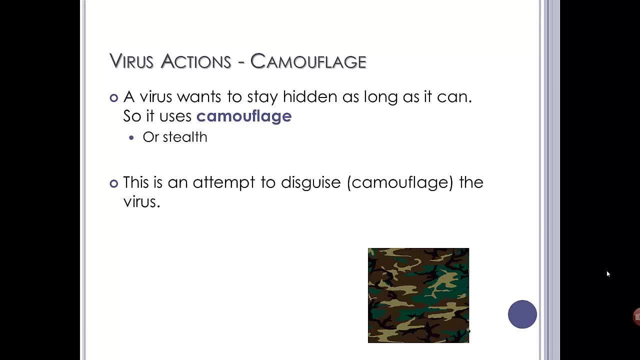 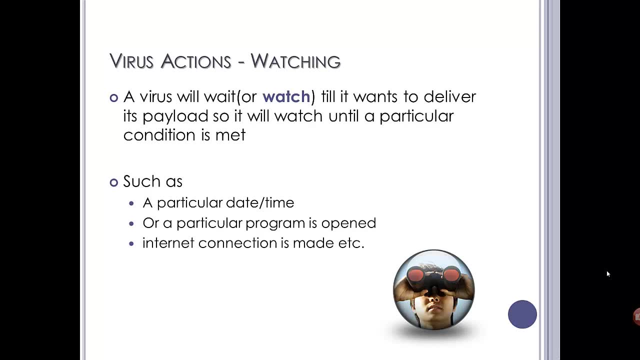 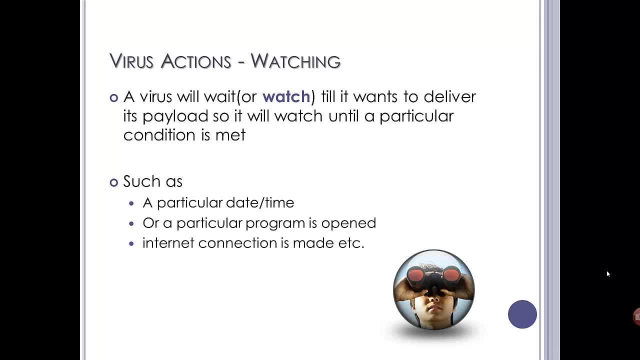 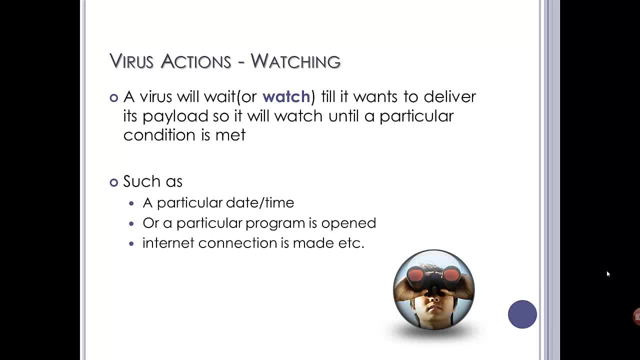 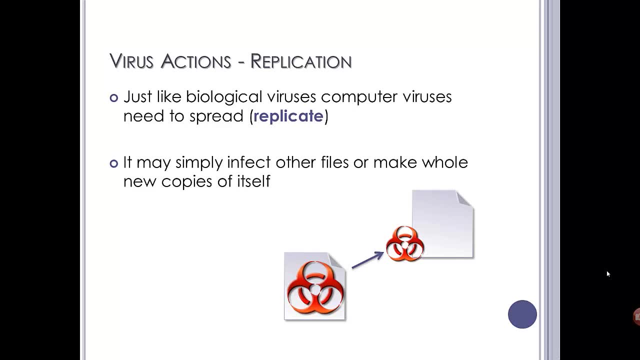 sit and watch until a particular event happens. Whilst it's doing that, or even after it's doing that, it may start to replicate. Now this usually means that it infects other files or just makes whole new copies of itself, So it may overwrite the contents of a legitimate 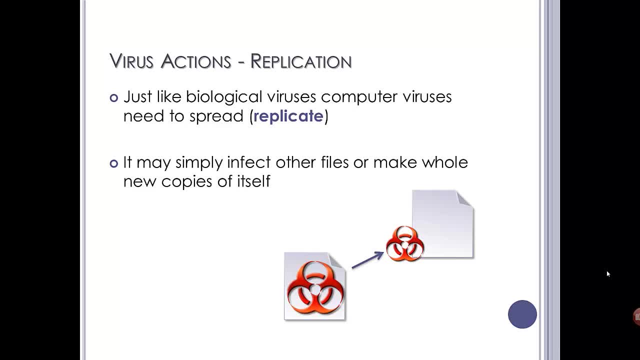 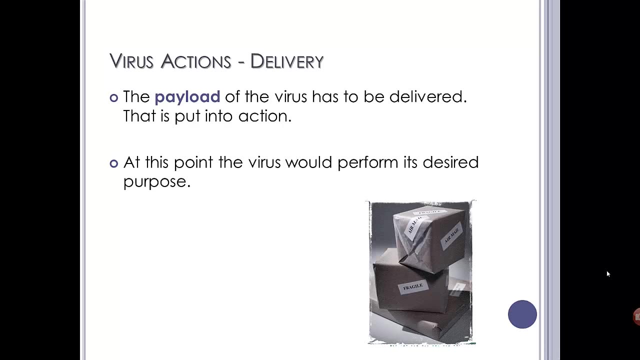 Word document, Excel sheet, or it may just actually clone itself and try and maybe mask itself as Windows-esque system files. And the last but not least, the delivery. This is when the actual payload, ie whatever the virus has been programmed to do so, whether 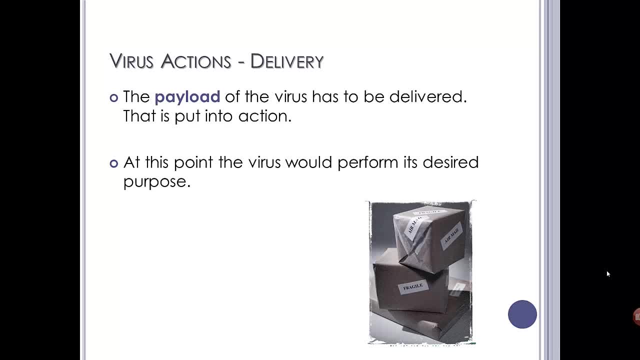 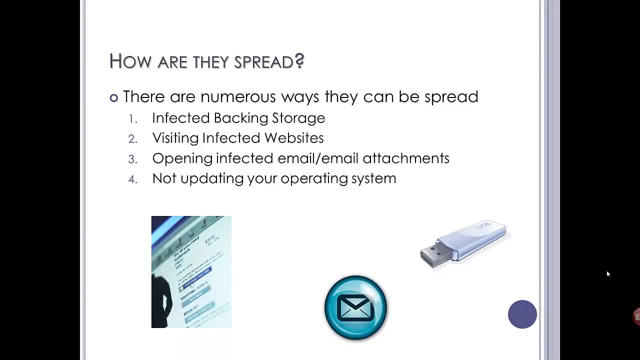 it's delete, modify, crash servers. this is when it would actually do its main task. So how are they spread? There are numerous ways they can be spread: Infected back-end storage such as USB flash drives, CDs, DVDs. Sometimes it's just enough to visit a compromised website. 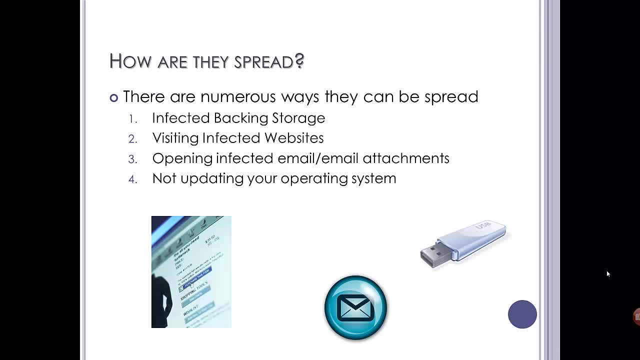 particularly if you've not applied any security updates to browsers, etc. Email opening affected email and email attachments can do it, And also just not updating your operating system or browser. When security vulnerabilities are picked up, it's fairly important, or it can be very important, that these are picked up and installed, or hackers. 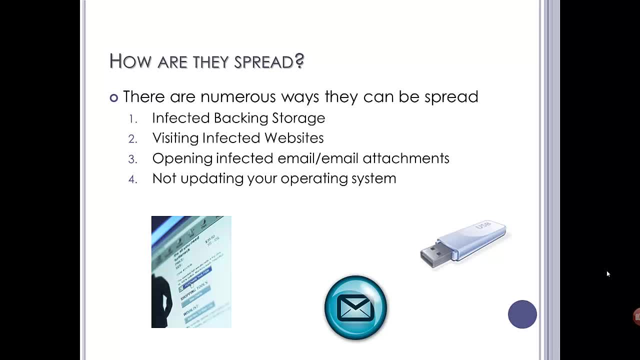 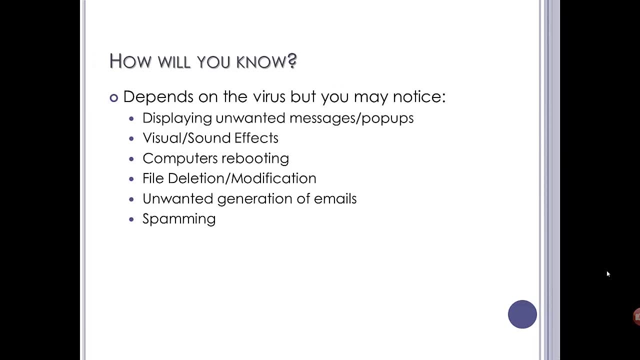 can utilise these to get a virus on your system. So how will you know? Oh, the best viruses may actually stay hidden, so you don't actually know. But what they can do is they can actually display some on-board messages, pop-ups. You may notice your operating system freezing. 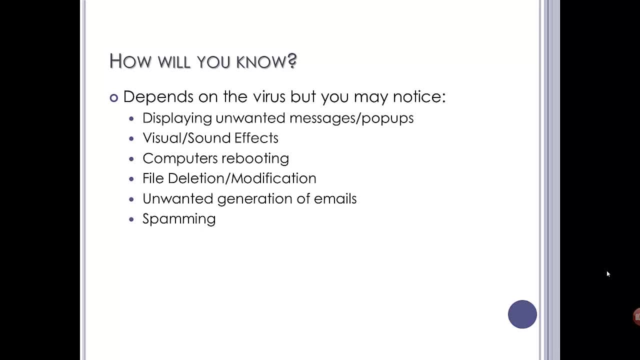 up locking up. a lot more Machines may reboot Visual and sound effects to a lesser degree. now Files may be deleted or modified, such as maybe Word documents overwritten, Windows sets and files altered. You might start. the last two points are kind of tied up there. 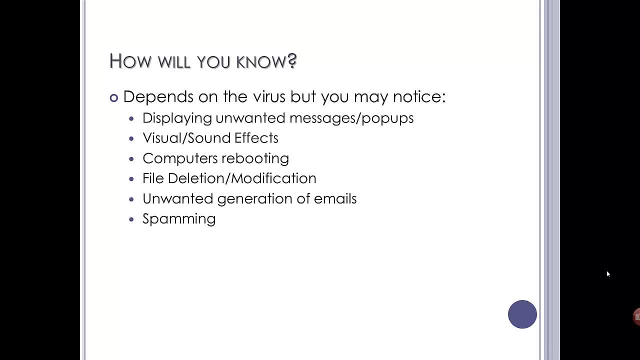 When you want a generation of emails and spamming, you might find that you're suddenly you're spamming your friends because you've been infected by a virus and that's what that virus does. So you may get a few emails from friends saying that you've sent them an email that 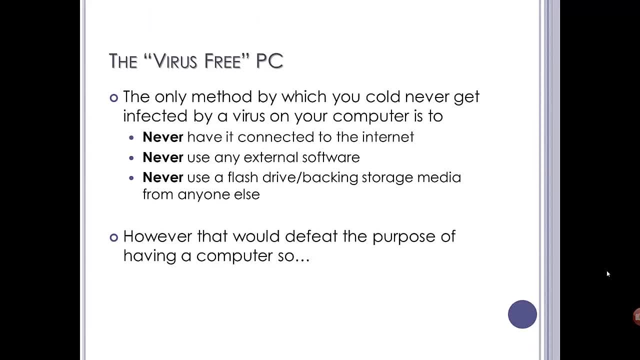 you have no idea about. The only way you could ever get a virus-free PC is it would never be connected to the internet, it would never use any external software and it would never use a flash drive or backing storage media from anybody else. That would kind of defeat. 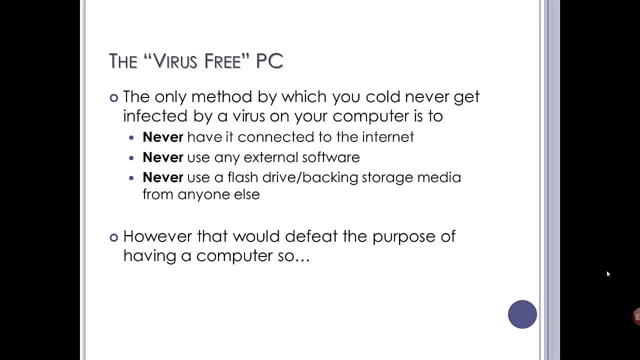 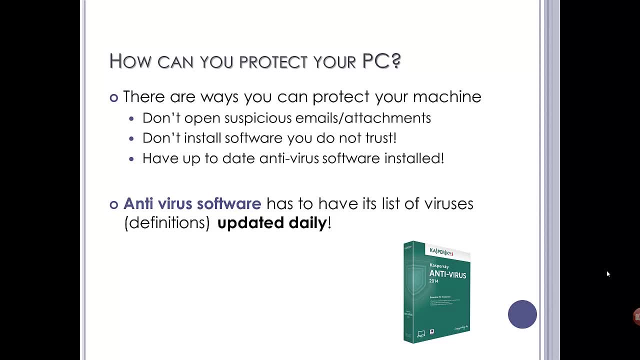 the purpose of having a computer, Particularly now. So how can you protect your PC? Well, there are a few ways. Before you install any software, you could just don't open any suspicious email attachments, even if it is from people you trust. You don't install software you don't trust If something 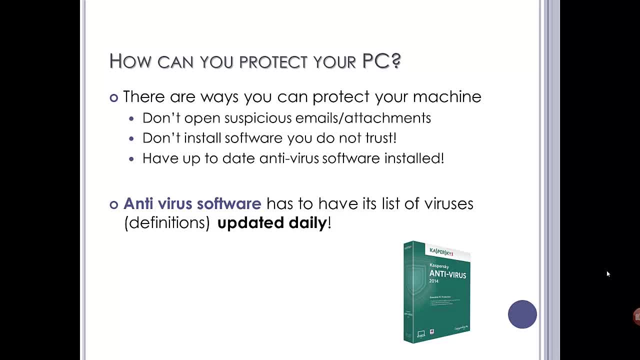 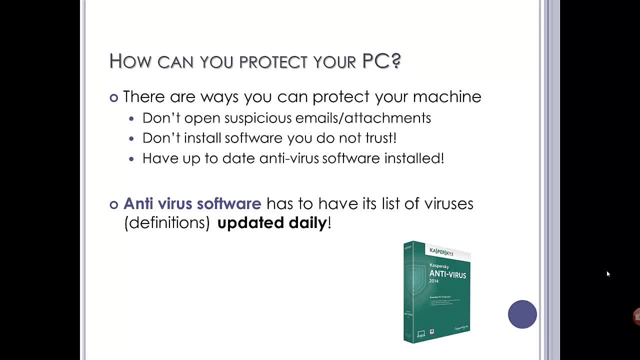 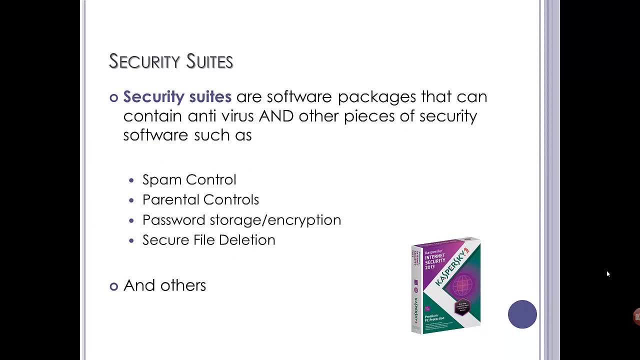 very good software. Anti-virus software has to have its list of viruses, all its information about viruses, updated daily. If you don't update those viruses definitions daily, it may not catch what they class as zero-day viruses or any of the newer ones As an upgrade. 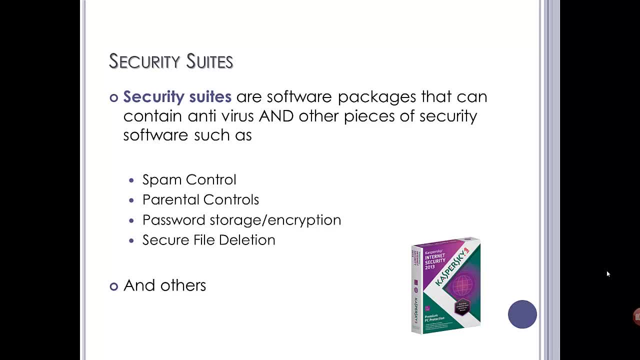 from an anti-virus software. there are security suites. These are software packages that contain anti-virus and other pieces of security software, such as spam controls, spam filters, parental controls, so you can filter out certain websites When internet connectivity is allowed, and such it can store and encrypt your passwords. 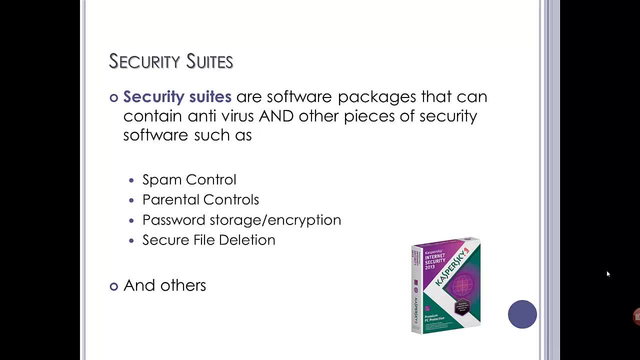 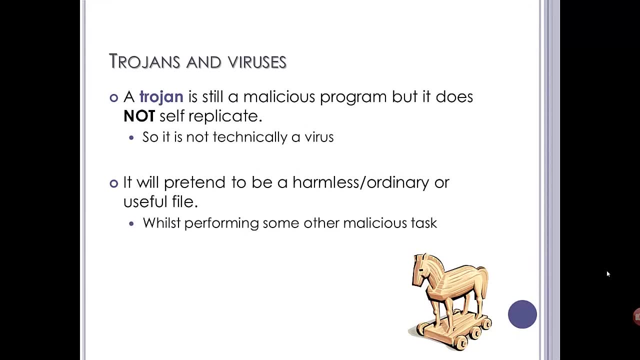 more on encryption later, and it can securely delete files, And there are lots and lots of other features that some security suites can offer. Now we've also mentioned Trojans. A Trojan is still a malicious program, but it does not self-replicate, so it isn't technically a virus. It will pretend to be a harmless. 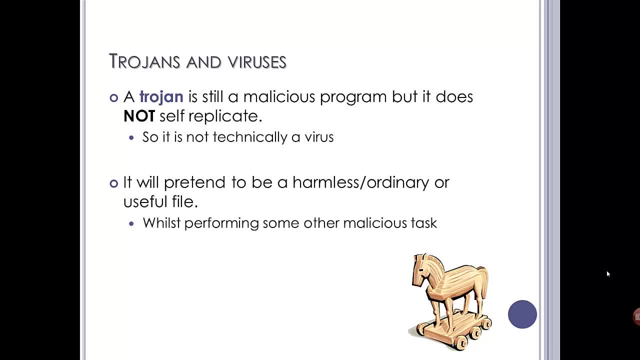 ordinary or useful file. Trojans can also be used as a virus-removal tool, For example. it might say it's a virus removal tool. It might actually remove the virus that it says, but in the process of doing that, install itself. 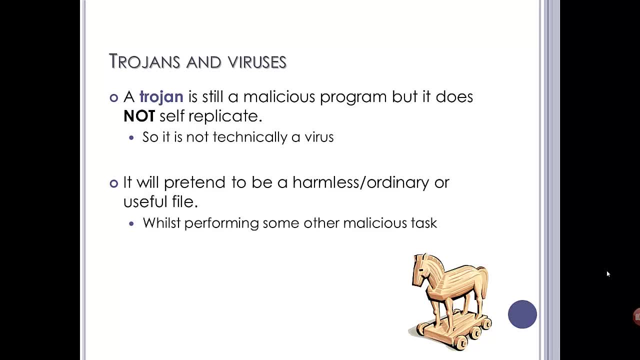 It comes from the mythological story of where two- I think it was Troy- and another ancient kind of civilization were at war. They woke up to find that one of them woke up to find there was a big Trojan horse outside the castle gates. They let it in and that night all 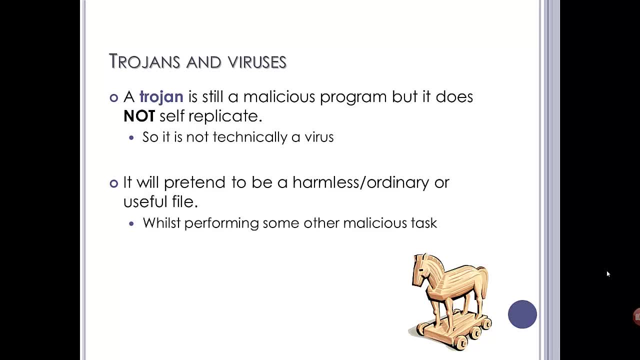 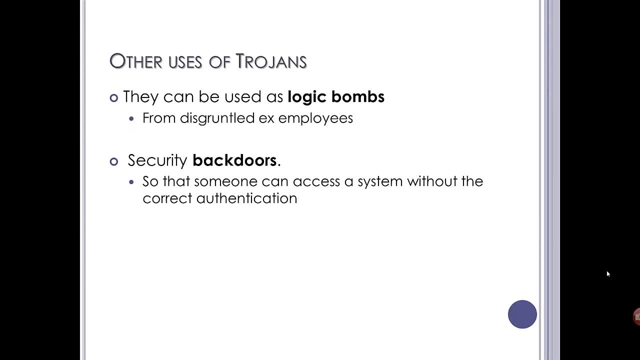 the soldiers crept out from the Trojan horse, So it looks to be a gift, It looks to be something promising, when it actually, in fact, does something malicious. Trojans can also be used as logic bombs. These are when it might go off a particular day. 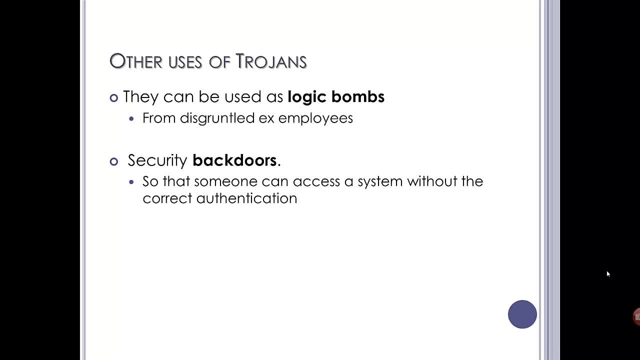 at a particular time usually cause kind of malicious problems And they can be used as security back doors. Someone can actually access a system without needing to go through the correct channels. Now Worm, Another form of malware that spreads via network connections. Now, these usually don't affect. 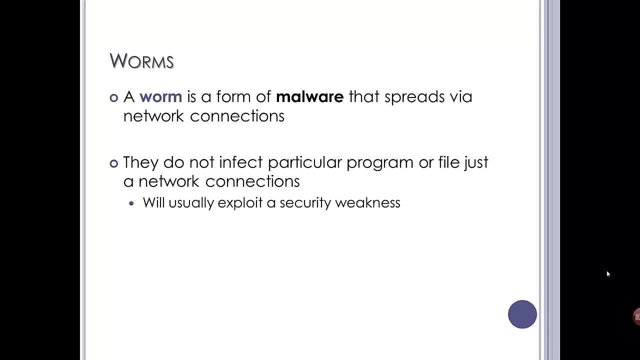 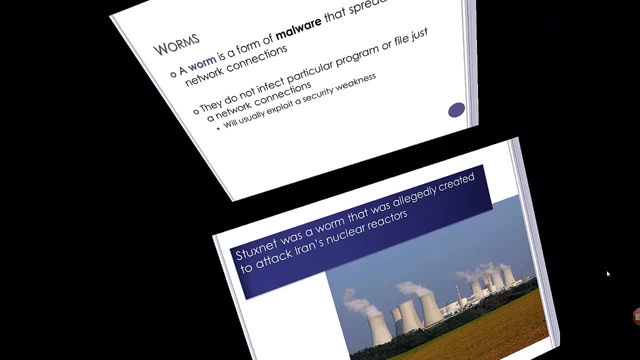 particular programs or files. They just need, want a network connection And usually exploit some kind of security weakness so they can spread themselves about. I mean Stuxnet, for example, is a worm that was allegedly created to attack Iran's nuclear. 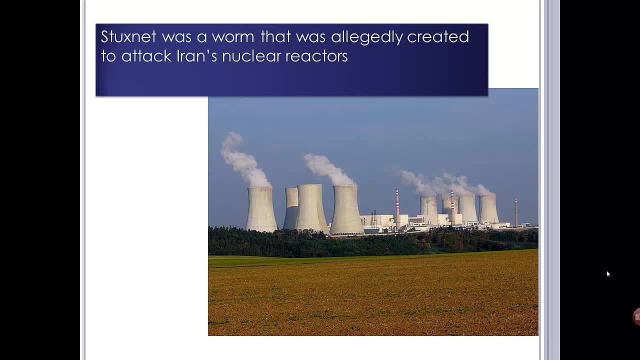 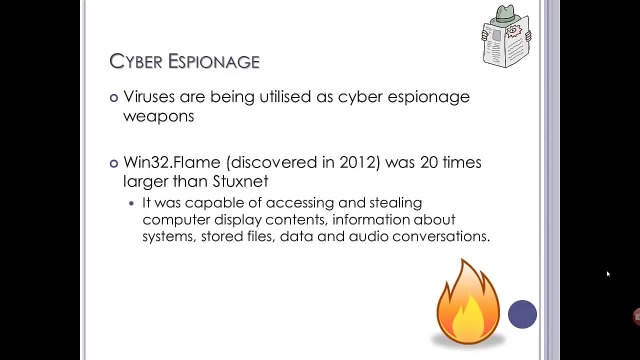 reactors. That isn't an Iranian nuclear reactor in the photo, but viruses are increasingly being used. It's been utilized as what we class as cyber espionage, cyber warfare. Think of the amount of your life that is controlled via a digital system, This Win32.flame, which means it's